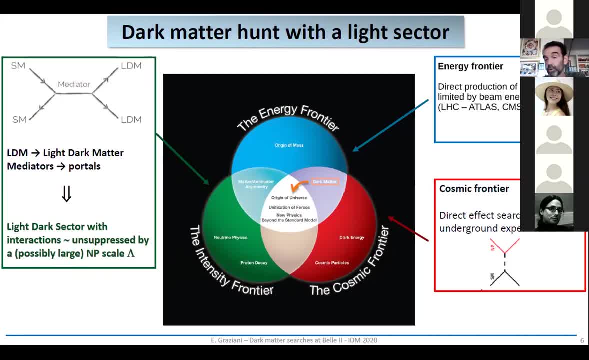 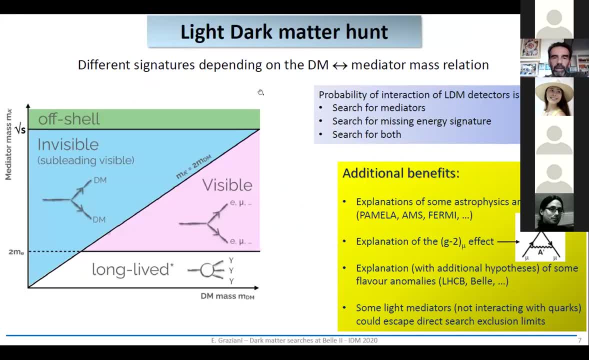 hypothetical large-scale new physics within reach or without or outside reach of LHC. Of course, whatever the dark matter is, light or heavy, the probability of interaction with the detectors is negligible. So what we really look for is mediators or missing energy signature or both, And we have different cases depending on 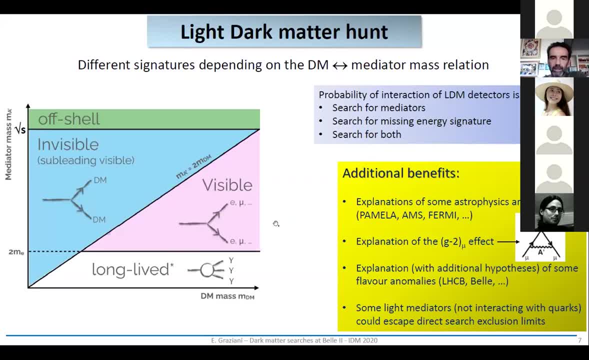 the mass relationship. So we have the relationship of dark matter with mediators: Visible if it can decays. the mediators can decay only to standard model particles, Invisible. in the opposite case, They can also be long-lived if mass are low or the coupling are tiny. 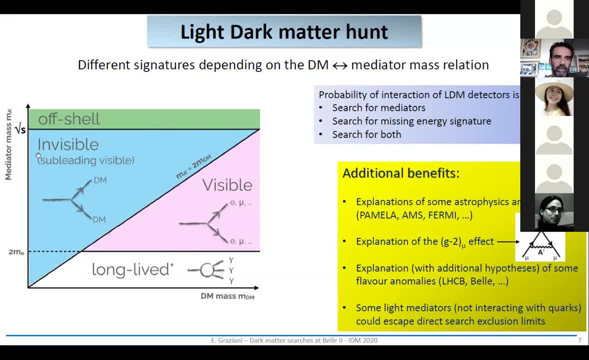 And the official case, which is the artist one, when the mass of the mediator is outside the square root of s of the machine. There are also additional benefits of having a light-dark sector, So we can explain astrophysics anomalies, the G-2, the anomalous G-2 of the muon. 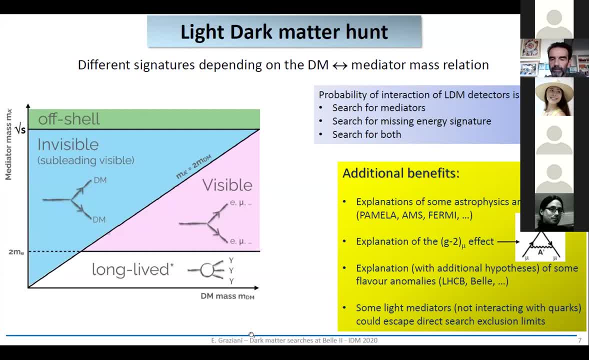 Also some flavor anomalies which will be our daily bread in next decades, And also the presence of light mediators could make limits from the direct exclusion, direct search experiment be escaped, because some of these mediators do not interact directly with the quarks and so with the nucleons. 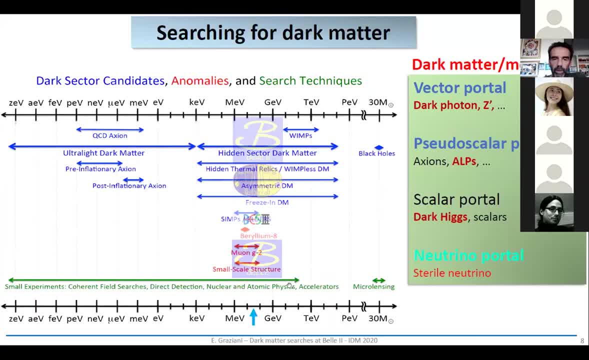 And of course we can't search for dark matter everywhere, but in this range, So from the MEB scale up to most or almost 10 GB, And usually these are this subdivision in classification of mediators according to their nature, in vector portal to the scalar, scalar or neutrino portal. 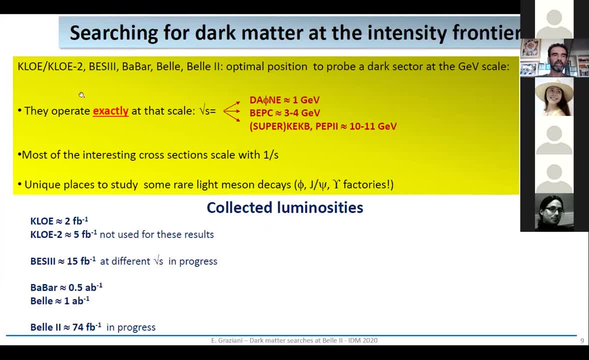 So, of course, if there is a light-dark sector in intensity experiment, high-intensity experiments are in the best position to probe it because they are working exactly at that scale. Daphne was working at around 1 GeV BEPSI at Tau-Charn threshold. 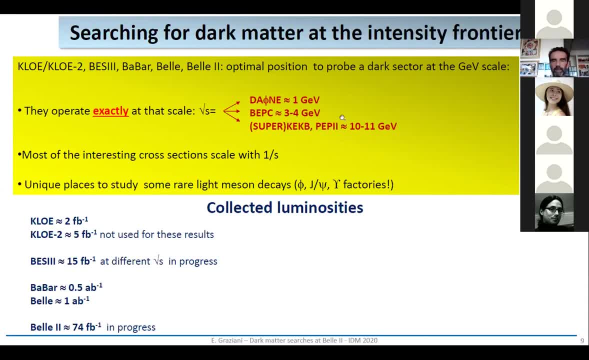 while Super-Keck-B Keck-B of course, and PEP2 around 4s, so at the bottom threshold. I mean we have to remind that most of the interesting cross-section scale like 1 over s, so there are very different situations. 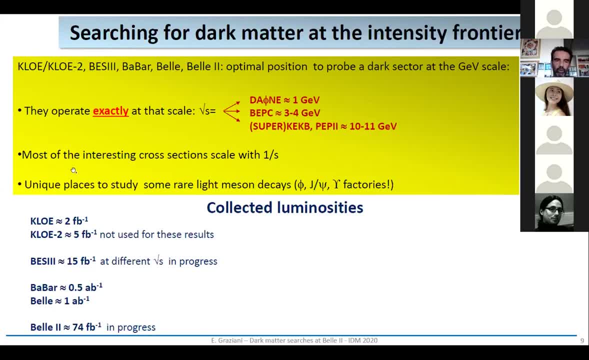 We need this machine with different machine, And these are also unique place to study some rare light-mason decays. because they are factory, they are supposed to do so Let's have a look at the collected luminosity by this experiment. In the past. CHLOE two inverse Phentobarn, additional five. 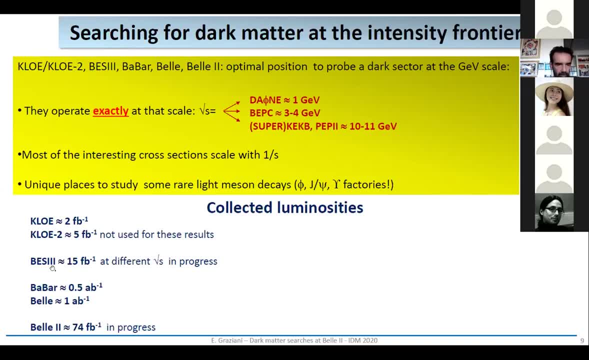 but still not used yet for this search: BES-3,, if I'm not wrong, something around 15 inverse Phentobarn, but a different square root of s. so different analysis, use, different integrated luminosities. BABAR: a little bit more than half inverse Atobarn. 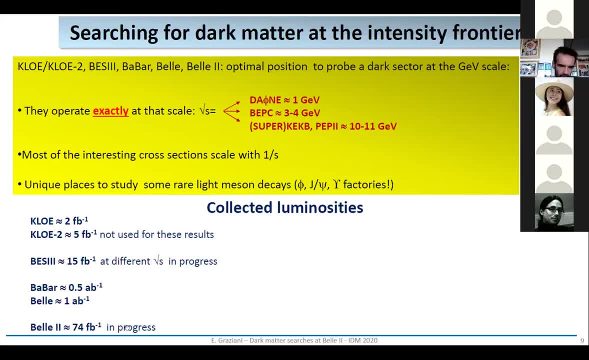 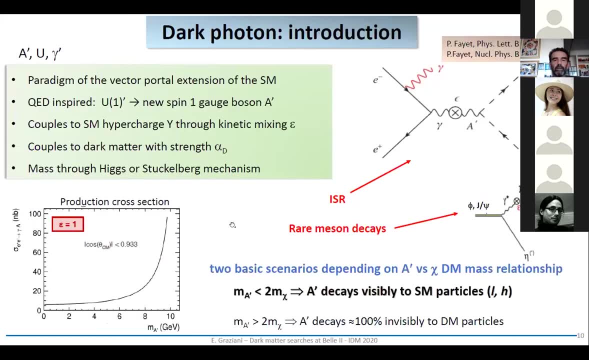 BELL, a little bit less than one inverse Atobarn, and BELL-2,, which is stronger in progress, collected almost 75 inverse Phentobarn up to now. So we start with which is a portal extension standard model. 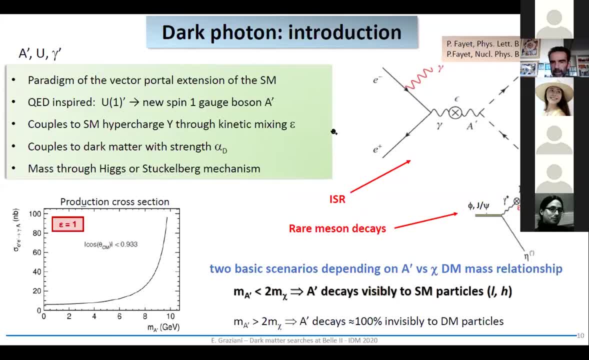 QD-inspired. one assumes the existence of a new spin-1 pitch boson which can couple with the standard model, with the charge standard model, through the kinetic mixing- this epsilon here- and to dark matter, with the coupling alpha-d. So again, two basic scenarios, depending on the mass. 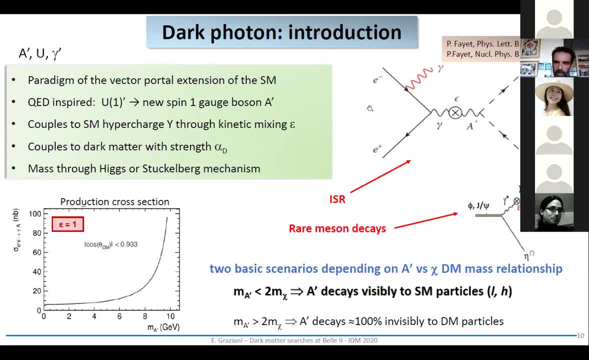 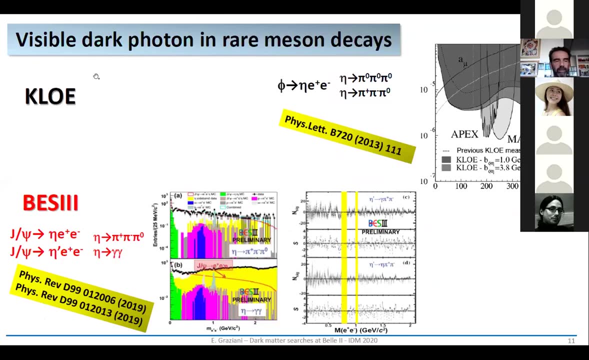 it can be visible or invisible At the plus-minus machine. there are two main ways of searching for it: in ISR processes or in ray meson decays, And the second one, the ray meson decays- CHLOE, for example. 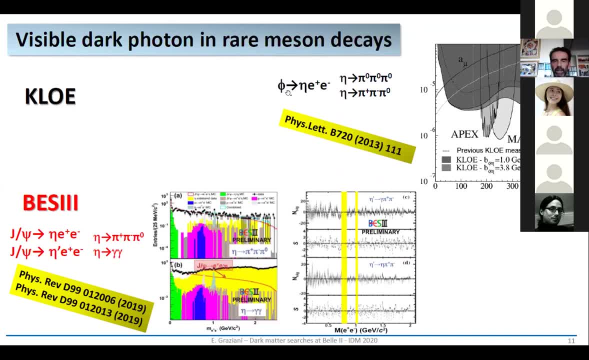 looked for a dark photon in the Phi to Eta plus-minus decay channel, with Eta into 3 pionts. That's a kind of exclusion plot. they got at the time of the publication, so that's some years ago. BEST-3 is pretty the same thing, but replacing the Phi with JPSI is natural for 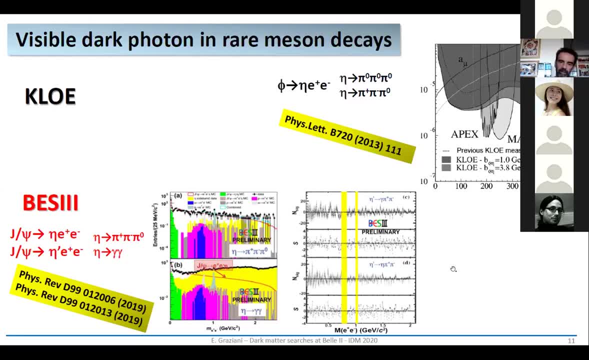 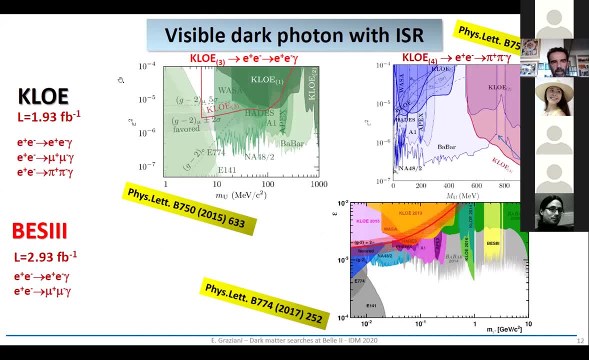 I mean given the nature of this experiment. Again, these are the results. The mostly used method was through ISR production. CHLOE did a quite complete job. I show you here. I light here only the most peculiar one in electrons. 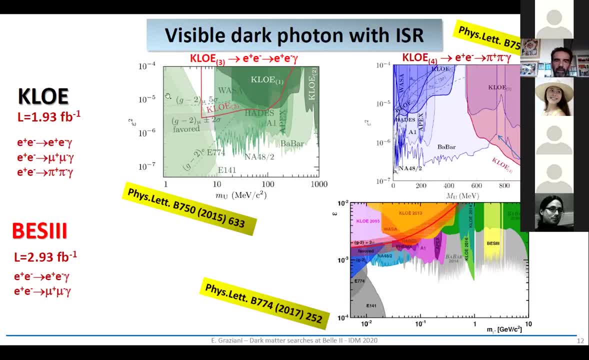 because they were able to go as low as 5 MeV mass And in pions they are still nowadays the only experiment. who looked for a dark photon in hadronic decay, For example? Babar here excluded the raw region from explicitly from the search. 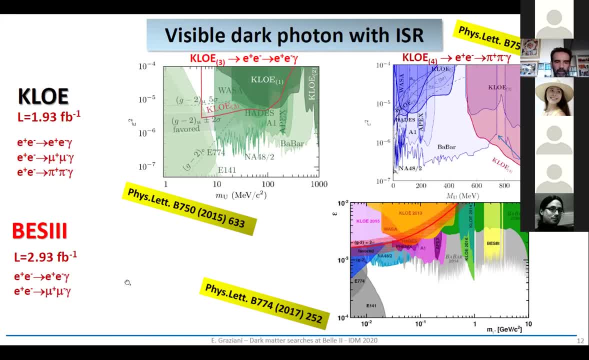 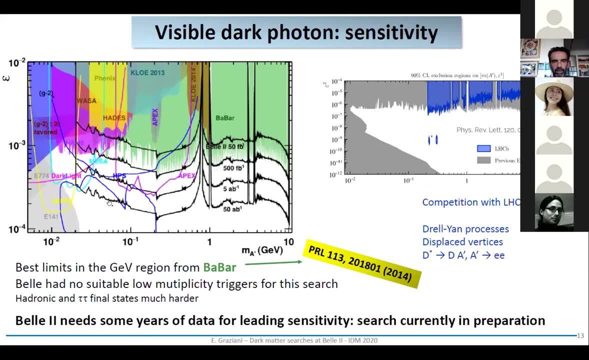 BEST-3, quite classic search, peak search for electrons and muon pairs with the photon. So ISR was really a worldwide effort. This is the current situation, with the addition of LHCb, which we also heard in the previous talk: The best limits as of now in the interesting region. 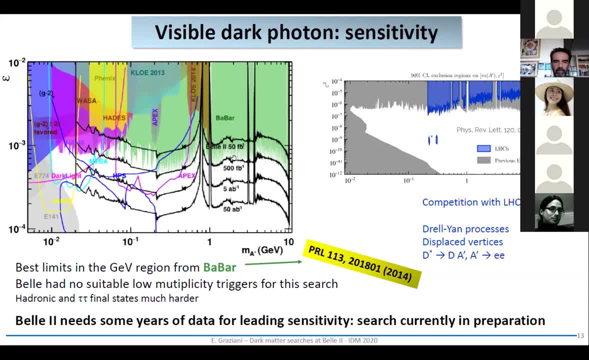 and so, at the GEV scale, let's say, are detained by Babar. BEST-3, quite classic search, peak search for electrons and muon pairs with the photon, The best limits as of now in the interesting region. and so at the GEV scale, let's say, are detained by Babar. 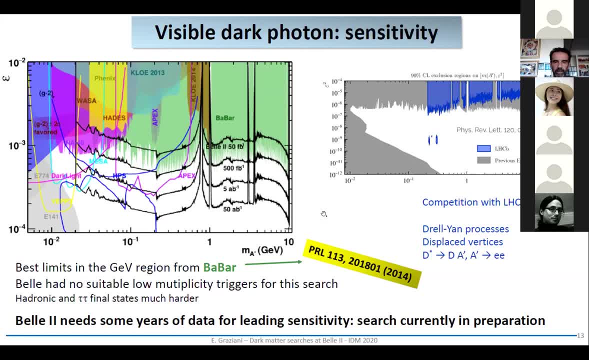 Bell had no suitable triggers for low multiplicity final states. Bell 2 has these triggers but still lacks some data, So this search is currently in preparation. When we will have data then we will really believe the sensitivity And of course, competition with LHCb is expected. 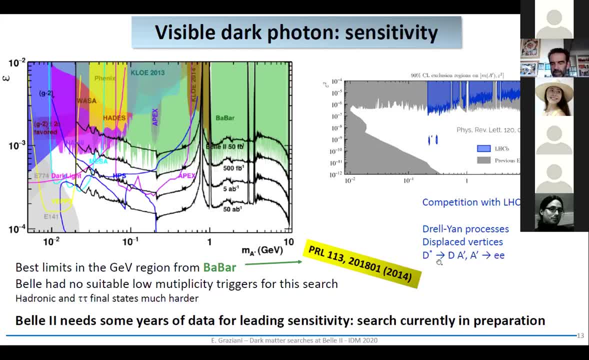 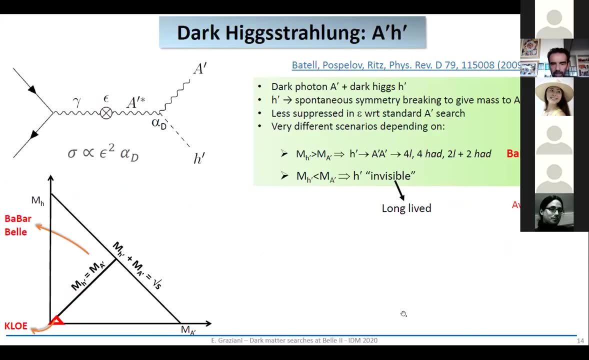 which we just heard in the previous talk, also because of this very interesting charm, decay with an impressive cross-section, at least seen on the scale of plus, c, minus interaction. another, another topology which was searched is the darking style. so here one tries to. the attempt is to give an answer to the question: where does the mass of? 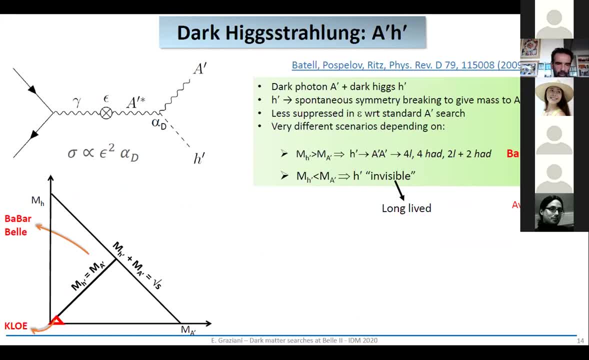 that photon come from, because it needs to be massive to explain the associated phenomenology. we know now since, uh, eight years or so that at least in one case- but a really important case- mother nature picked up the spontaneous symmetry breaking mechanism. so we what? what we imagine here? 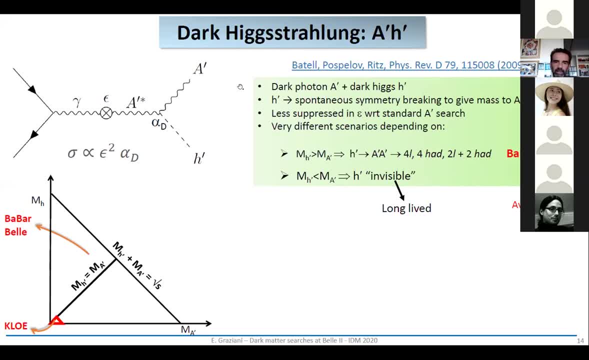 is again in analogy. uh, we assume the existence of the darkings at h prime and again the phenomenology depends on the mass relation. for x, uh, heavy x, it can decays to two dark photons, so that that's the equivalent of x to gamma. gamma decay in the standard model for a total of six charge particle. 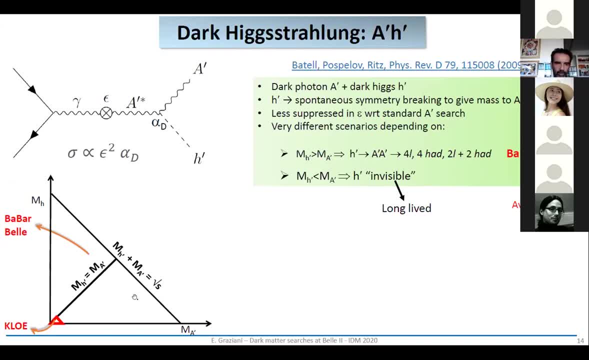 so this is a truly two-dimensional search, because two particles at the same time, two peaks in the, in the, in the two mass, and in this case one would populate this region of phase space, while in the complementary case is for a light, x. so in this case it would be invisible rather than invisible. 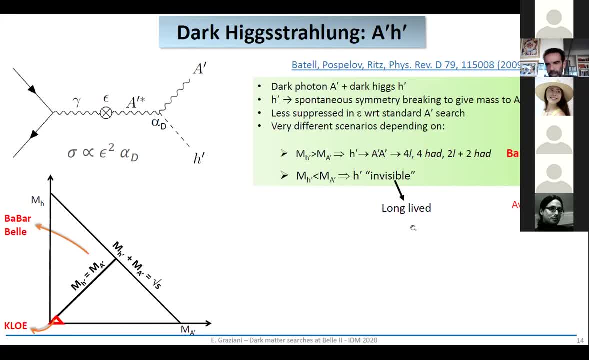 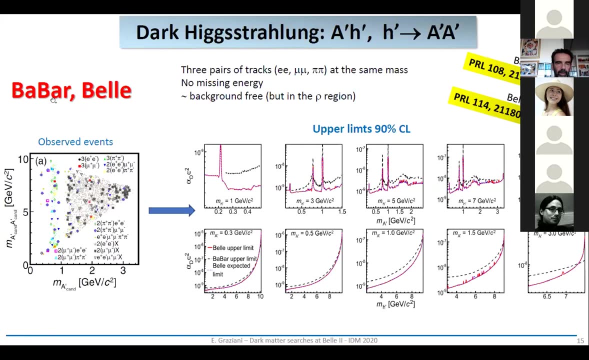 long lead, so with such a long lifetime as to decay after outside the detector. and this was searched by chloe, in the limit, of course, uh allowed by by the, by daphne energy. so the first case about in bale, this is the final spectrum for 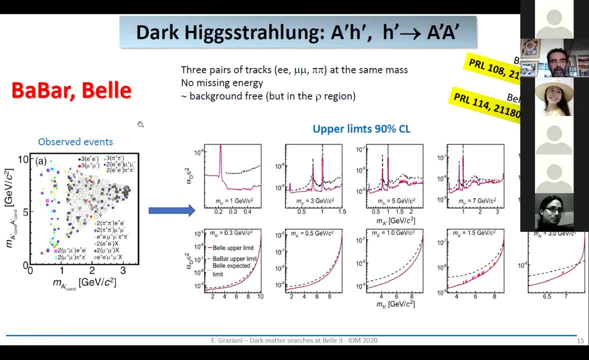 bell. you recognize here the triangular shape. it's a. you expect a very clean signature, three pairs of tracks each at the same mass and staying on the forest, so no missing energy. very, very clean signature, almost background free measurement which reflects into the limits you can set to the couplings. by the way, 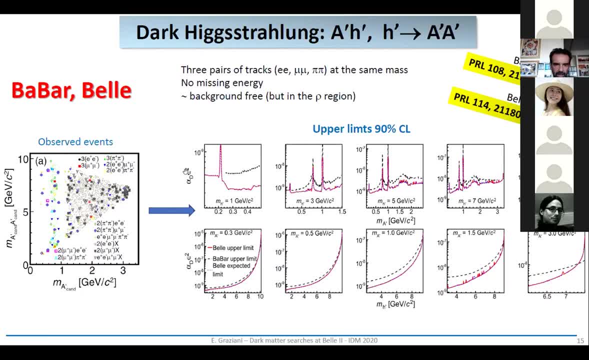 the couplings is not simply epsilon epsilon square, but it's alpha, dark time epsilon square because there is a dependence on the coupling constant. so usually one um one displays limit, fixing one mass x in this case, and looking at the upper limit as a function of the other. you see here bell and babar. 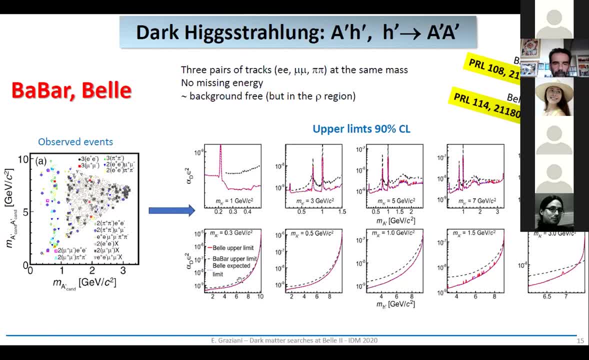 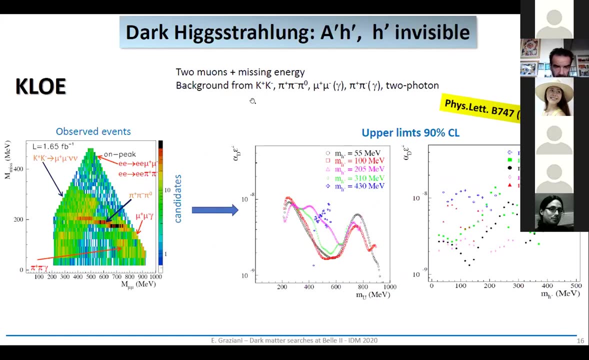 and here the other way around. um numerically limits between 10 to the minus 8 and 10 to the minus 9 in alpha d times epsilon square. complementary case by chloe, two muons, a missing energy signature. this is not a background free measurement. it gets background from charge. 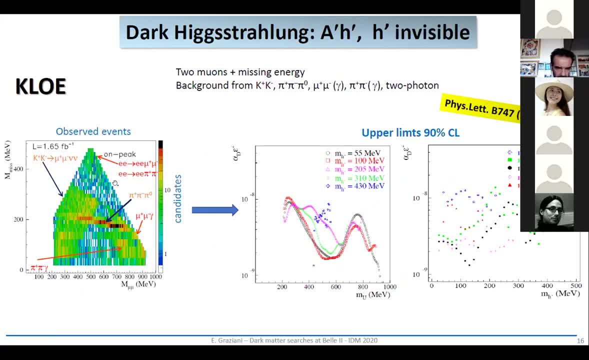 chaos and three pions and the limit, that's the final spectrum, and the limits you get are here again, one must best fixing, fixing one mass and let's say, in the looking at the other same numerical limits, 10 to minus 8, 10 to minus 9. of course they can, they cannot be combined, superimposed. 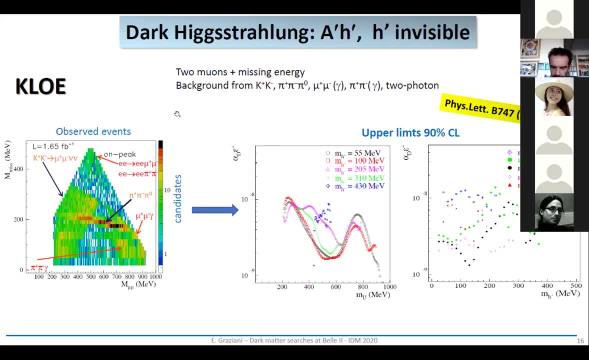 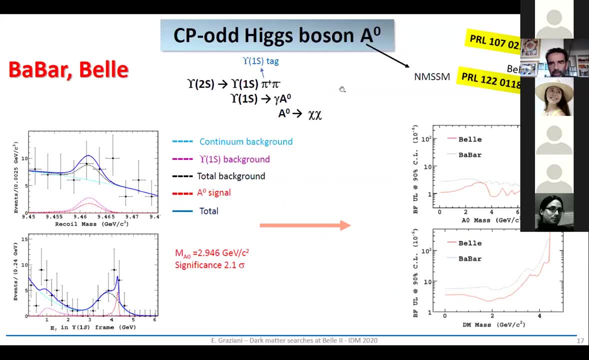 with that, with those from, because they belong to different, to different phase space. another search: uh, that's just an highlight so that not all, not at all all, the searches have been performed. this is the cpo, the search for an x boson a0 which came out from some non-minimalist. 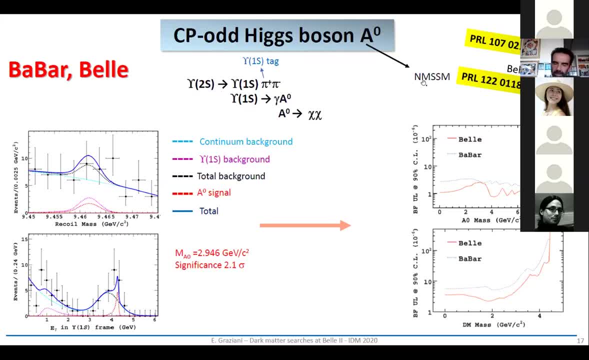 supersymmetric extension of the thunder model. in this case one looks for this a0 in the decay chain 2s, which means actually running the pep2 or kkb at the 2s and not as usual at 4s, so decaying into 1s and 2 pions which tag the presence of 1s, and 1s is supposed to decay into a photon and this a0 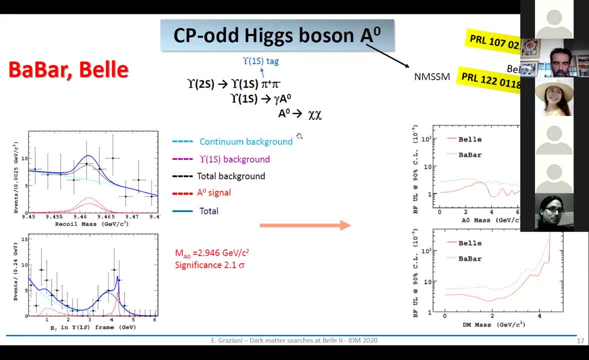 the a0 and dark matter, so invisible. so two variables: the missing record mass, which tags the 1s, and the energy of the photon, which is related to the mass of the a0. so this is an example and the best significance got by bel, which is not significant at all, of course, and the limit by bel and babar for this a0. 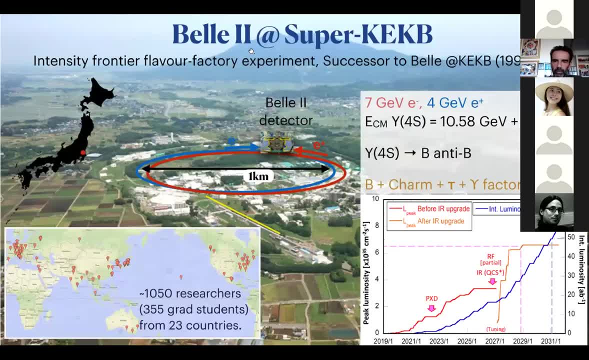 so we come now to belt. i mean, everybody knows that is the successor of bell, which was successfully running in the first decade in the mass load, interest and distribution value benchmark- almost decade, millennium. but two is a big experiment: more than 1 000 members, more than 100 institutions. 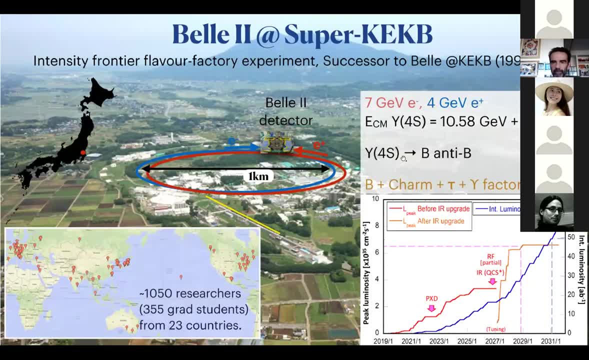 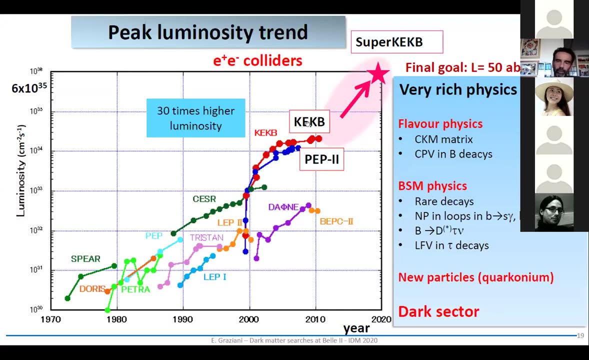 so again, it's an asymmetric b factory and with an aggressive luminosity profile. you can see this. here we are, in the instantaneous luminosity across history in the last half century. we are here, this last step, which accounts for a factor 30 in instantaneous luminosity, with the 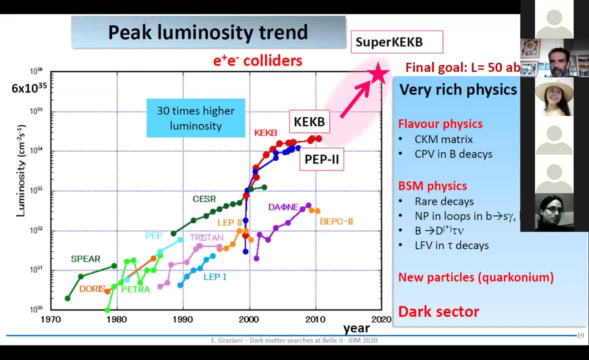 final goal of 50 in versatobar in 10 years from now, which is a factor 50 above bell. to this corresponds a very rich physics program which is of course centered around the flavor physics but does not neglect at all that set of search. that's quite technical: how to go from kkb to super. 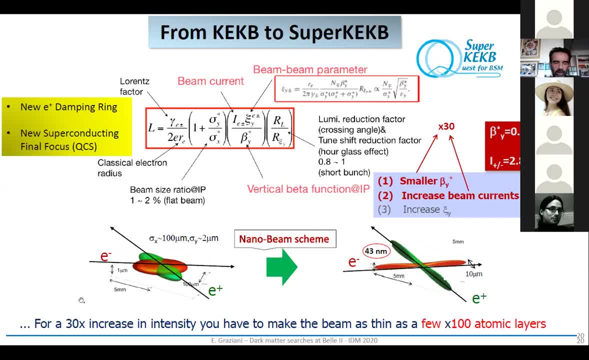 cake b. so how to make out this factor 30 in a word, there is a keyword for this: nano beam scheme, which means roughly reducing the size of the limit interaction point you see visually here, and also some contribution from an increase of beam currency, not extreme. so together they make. 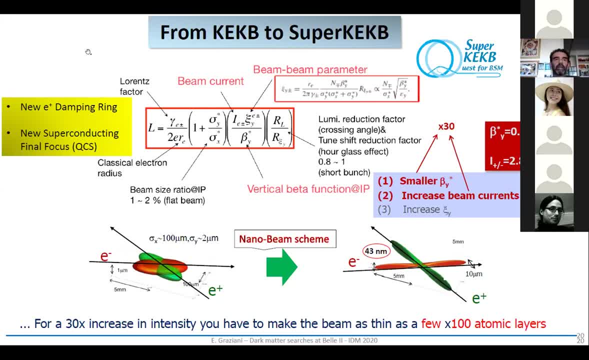 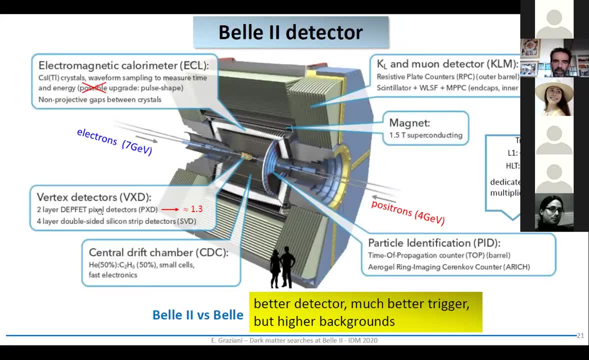 this factor 30.. well, to detector is a strongly upgraded these brand detectors in the internal part, with the new vertex detector, two layers of peaks cell- unfortunately one is incomplete- and four layers of strips. a drift chamber which is bigger than that of bell. a new particle identification system. type of propagation counter in the barrel. 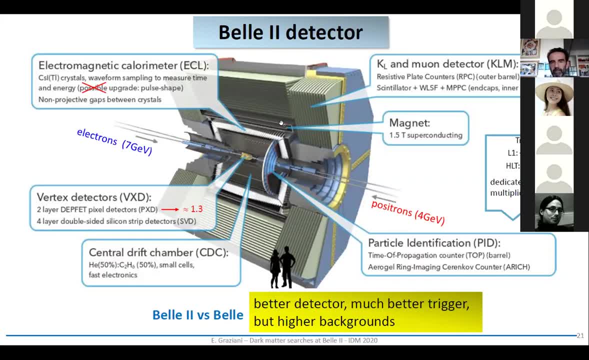 and aerogel in the forward, in the end cap, same magnet as in bell, same structure for the calorimeter and for the immune system, both with the brand new electronics. in case of klm, the active detector used to be rpc. now they are partly replaced by scintillators in the barrel and fully. 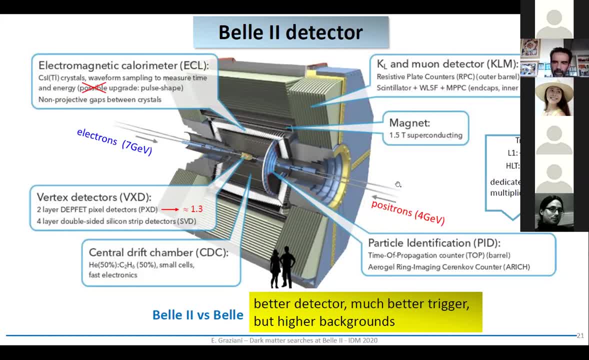 replaced by scintillators in the in the head cap and- that's important- new triggers with dedicated lines for low multiplicity physics. this was not the case in value, so overall level 2 is a better detector with much better trigger. unfortunately it will have to face worse background condition due. 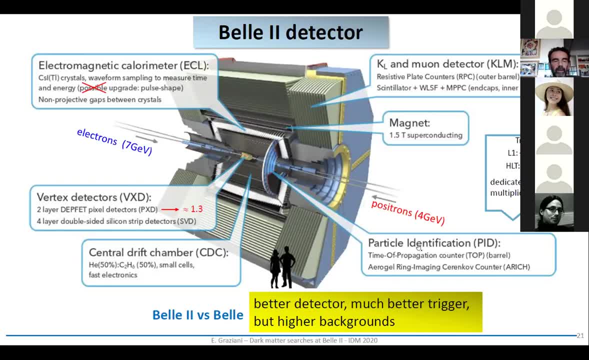 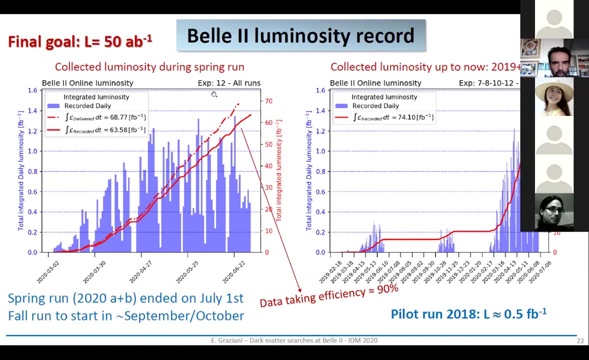 to increase of luminosity, and just talking about luminosity, this is what we win- have been able to do up to now: collect during 2020 we collected almost a 65 in west fentoban. the run- spring run- finished on july 1st and we'll take 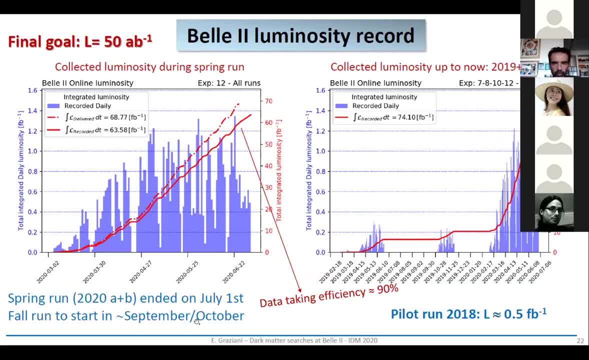 again, or the full run in uh beginning of october, probably overall, including also 2019 data, we have collected about 75 in perspective, to which you have to add the pilot run two years ago, 2018, which is quantitatively moving alpha investment, but but 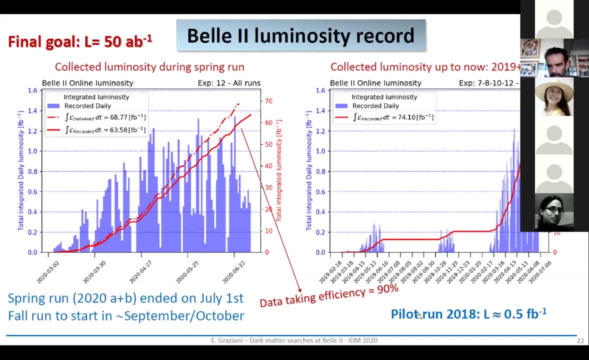 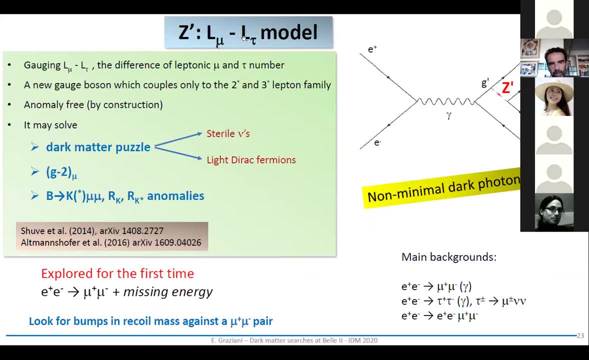 relatively very important, because two physics paper came out from this small sample. so the first model we checked is the new minus cell tau model z, prime. again one gauge: here it's a no minimal dark photon, because here what is gauged is difference of leptonic, new and 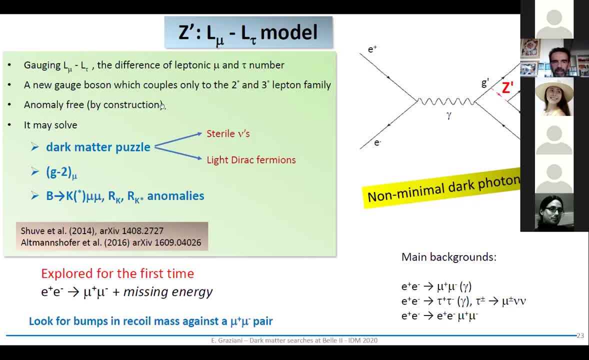 number and because of this difference of course one gets anomaly free by construction and couplings only to muon and tau. so it can be produced only as a final state radiation from a muon or tau leg in in the plus minus conditions. that's also enough miracle because in principle one can. 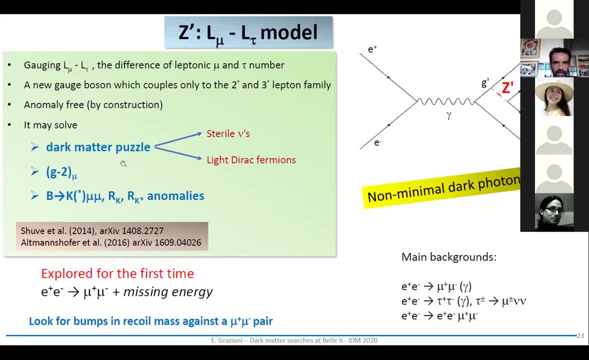 solve the dark matter puzzle, so predicting the correct relic abundance, with two different methods. by the way, with two different scenarios, two different dark matter candidates. there are new three nodes, in one case only light direct fermions, in another case. but you so? they are two different models but identical from the mediator point of view, and also the g minus two are the muons and 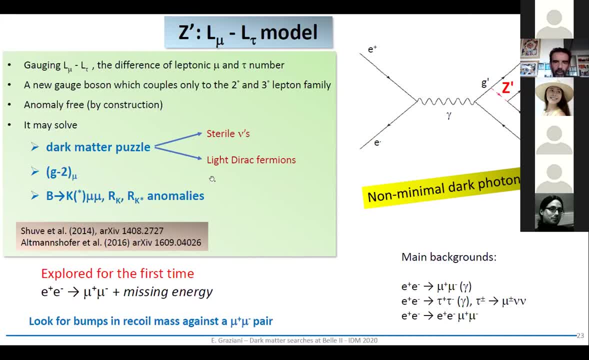 with additional assumption also the flavor anomalies. so in betu we analyze for the first time, we search for the first time the presence of an invisible z prime decaying to neutrinos or, even more interesting, to dark matter. signature is two muons and missing energy with the, with the, 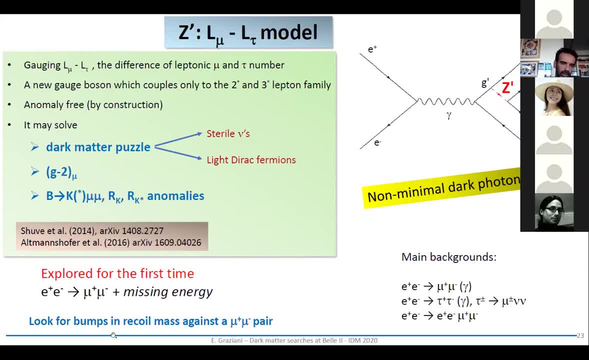 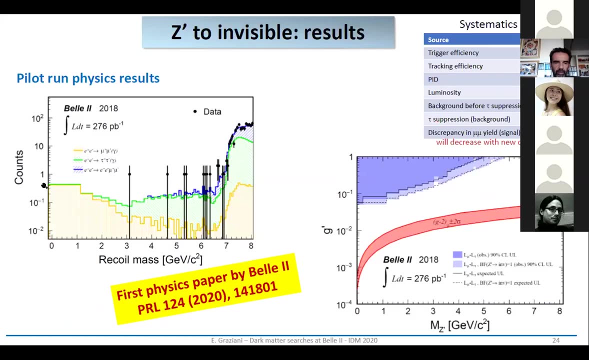 system recording against two muons peaking somewhere. main backgrounds are qd process with which produce muons, and missing energy in the final state for most of the space of the mass space. this is a background free measurement, the the sample which was used was the pilot run. 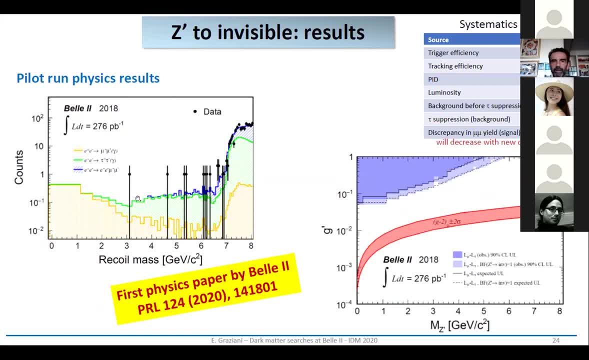 in alpha pilot run because of some problem in the trigger. so this data went into our fist. first physics paper publication, pls two months ago, three months ago, and this is the final limit we got. we are a bit. in terms of the coupling constant, we are a bit. 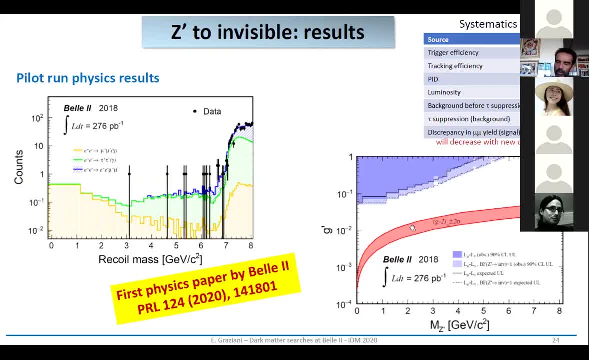 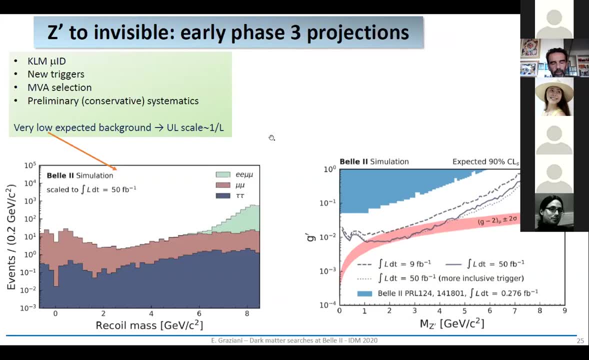 far from the g-2, but the expectation is to fill this gap soon. in fact, we have already projections for the luminosity that we have already on tape, but actually we have more than this that it will be a new analysis with, because of course, in the pilot run, the 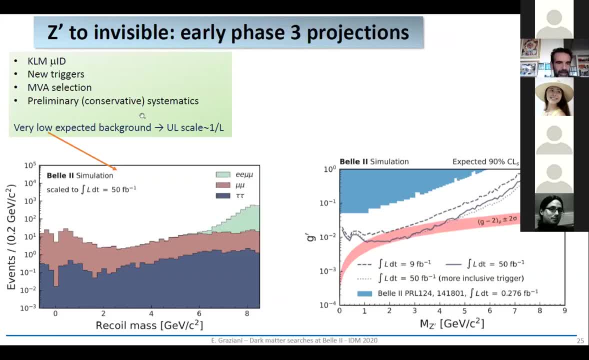 conditions were dirty and the heroically faced. but now we are in another phase. it will still be, as you can see here, this, this is the background expected: a very low background measurement, almost zero. so the limits are expected to scale like luminosity and not square root, and we are expected to probe seriously. 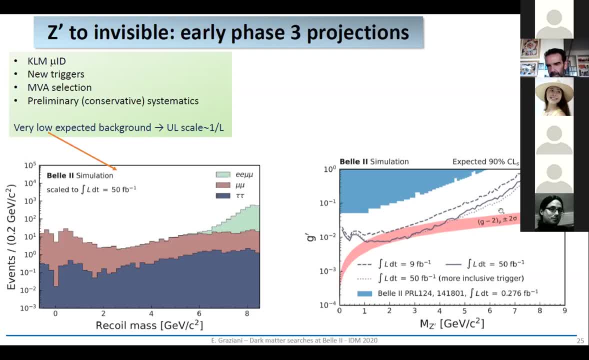 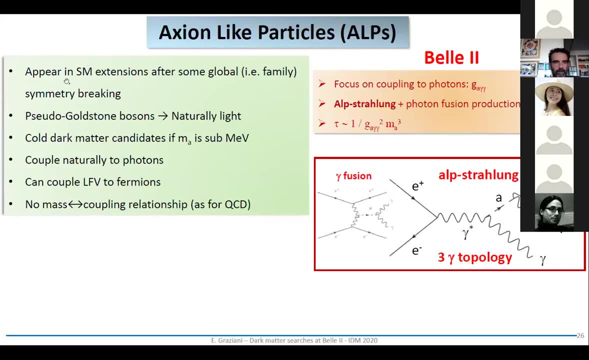 g minus to bend, also with the additional dedicated triggers, even better at high mass. second step is the action light particles, which are which appear in many extension standard model whenever a global symmetry- and family, family flavor symmetry is a good example- gets broken, so they come out as a pseudo-golston boson. 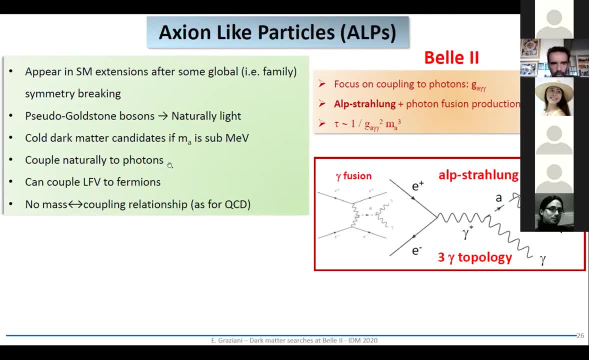 and because of this they are naturally light. they initially couple to photons, to bosons in general. a simple and typically from the qcd actions, the uh, i mean the one queen mpc long time ago. there is no direct relation between mass and coupling. so in in belt tool we focus. 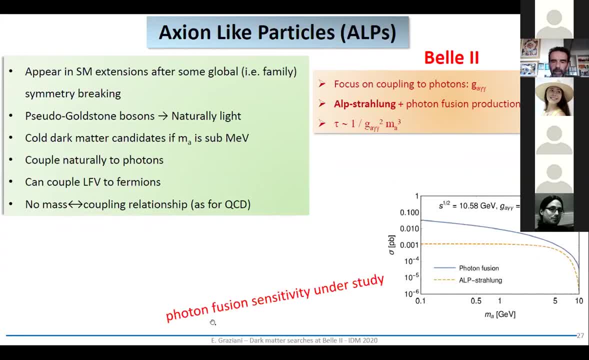 coupling to photons and we have two main production mechanisms: the extra long ended gamma fusion and um. even if the gamma fusion to fourth is lossводing when it is noses is losing tão two photon final state is favorable from the cross-section point of view. It's not so from the detection point of view. 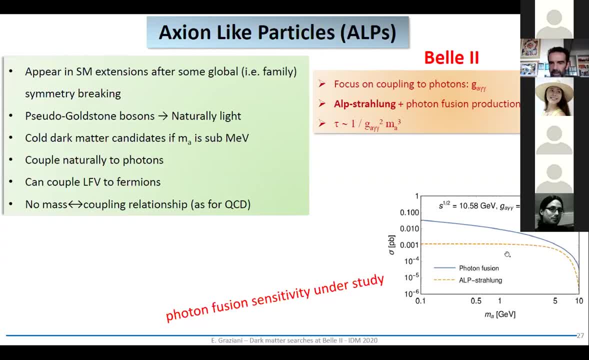 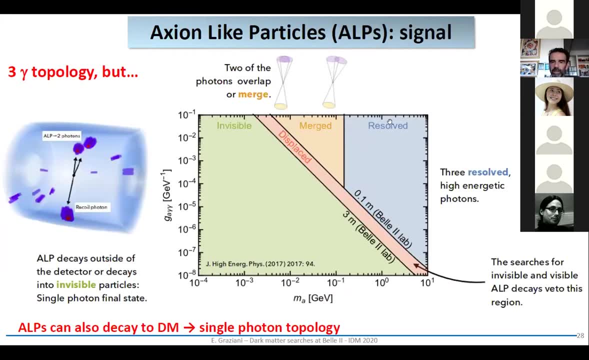 that this topology is easier, is cleaner, And so we focused on the abstract topology in the result case, which is what we faced in the two. But life is not is harder sometimes. So there are cases for low masses of the action light. 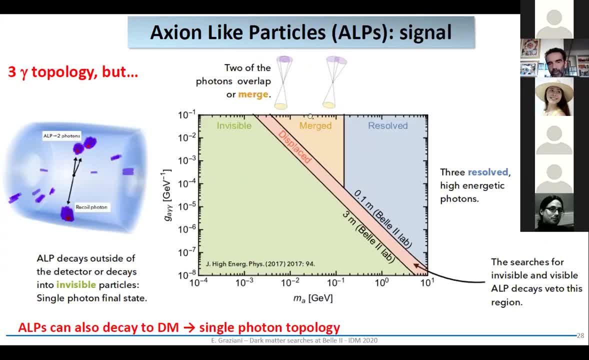 particle when the two photons are so close that the calorimeter cannot disentangle them anymore, And so this show up as a two photon topology, And the worst thing is that the worst case is that it can be suppressed at the trigger level if some veto for the standard model. 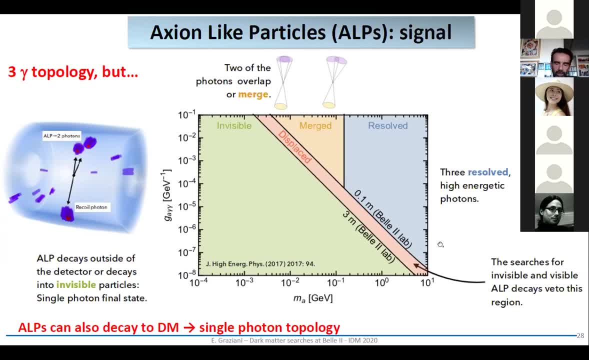 the plus minus to gamma gamma process, which is a high cross-section, is enforced. It's not the case yet, but in the future it's not excluded. Another case is when, either because of the mass of the particle- low mass- or because of the low coupling. 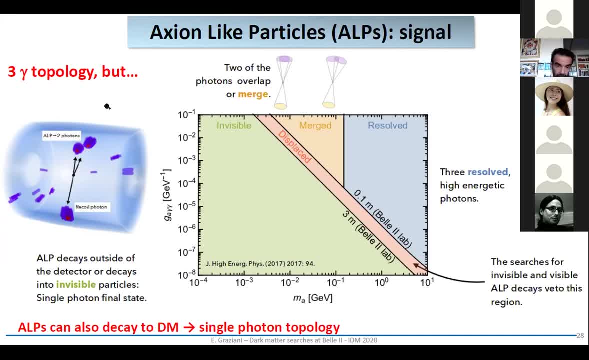 the particle gets enough lifetime to decay outside of the detector and one is left with only the recall photon. So one photon, single photon topology, which is shared also by the case in which this particle can decay, to that matter. So we have one, two and three photon topology. 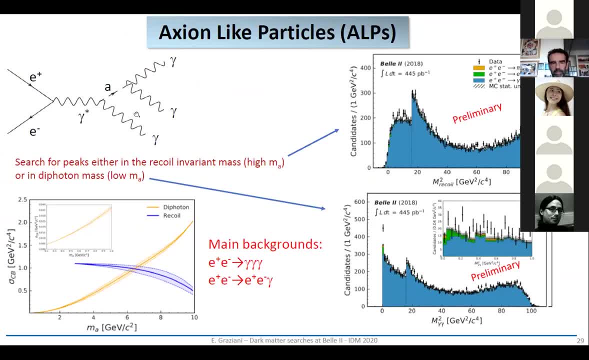 In the two by now. we just search the three photon topology, the cleanest one, by looking at the peaks either in the photon mass system or in the system recording as this isolated photon I mean different masses at different resolution. You see, there is a turning point where one method 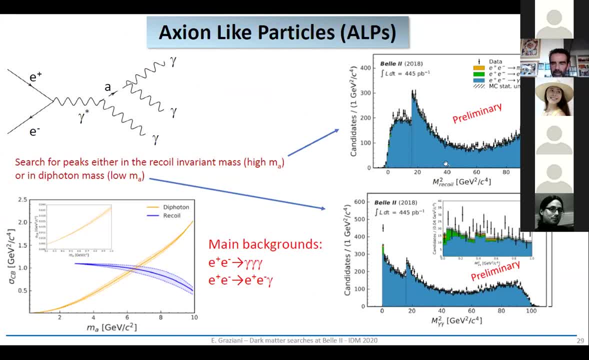 is more convenient than the other. So we study both the spectrum recoil and direct And this is the data compared as Monte Carlo. So if you are jumping on the chair because of this, you can sit down quietly, because if you look at zoomed, with a smaller scale, 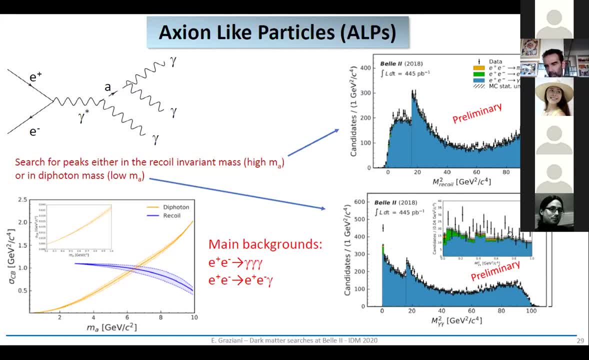 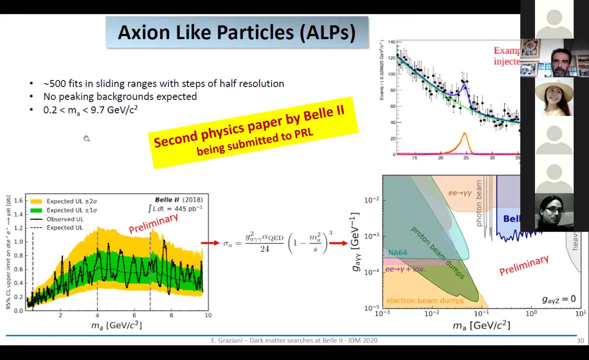 then you see that this does not appear really as a peak, but it's a quite diffused excess which probably point to some trivial issue in the Monte Carlo, in the simulation. but certainly not a peak, not a real peak. So this was the subject of our second physics paper. 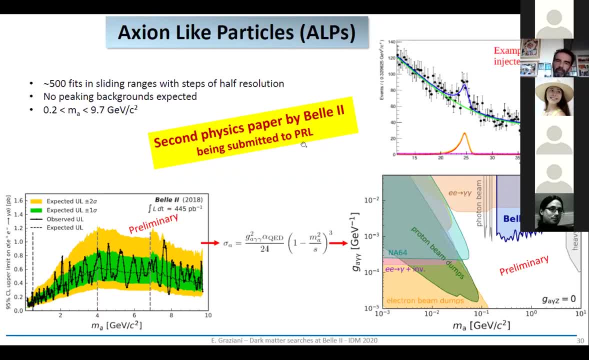 by Bell two, which will be submitted to physical review letters in a matter of days. These are the limits which we observed as usual, compared to expected, translated in terms of the coupling. So this is the first time this I mean. 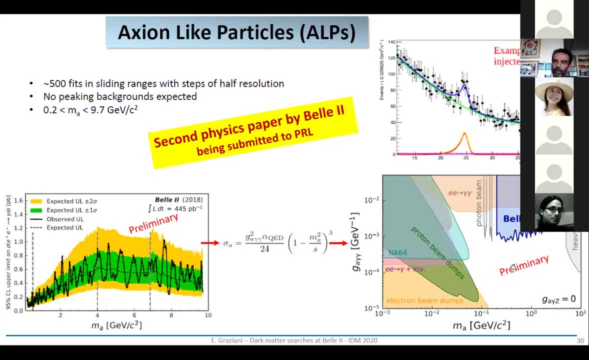 this is presented in this conference. I mean worldwide. So you see that we set the limits which are in our range, even one order of magnitude better than the previous one: E, gamma, gamma. it's essentially like: yeah, these are coming from that. 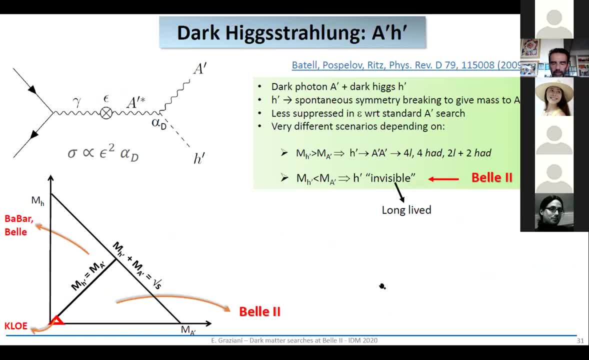 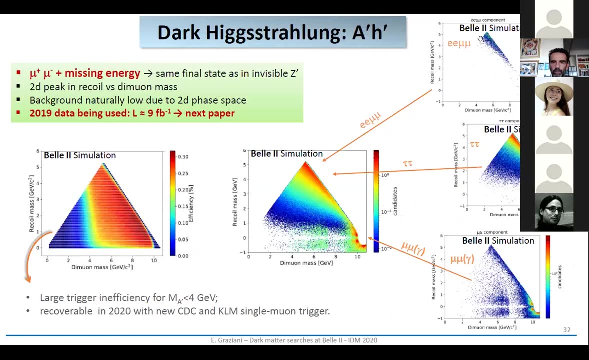 Also, we plan to use the to search for Dark-Egg-Stallaron process in the Chloe fashion- let's say So here in this region- for lighter. it's boson So in this triangle. That's why you see all the triangle now appearing. 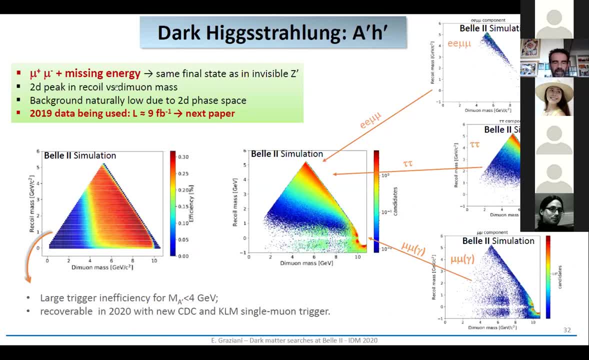 the two mass, one versus the other. It's the same final state as for the Z prime two mu and the missing energy. So the same background source are contributing And you see how differently they populate the phase space. This is the efficiency. 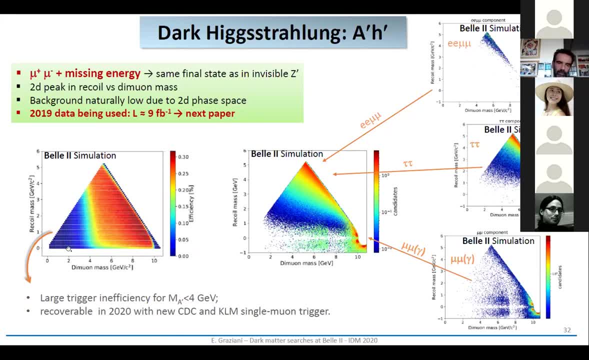 You see here a problem: We are almost blind for light dark photo masses. This is due to inefficiency of the trigger, which is cured this year in the specific dedicated tracking trigger and also with the introduction or KLM single-nual trigger. 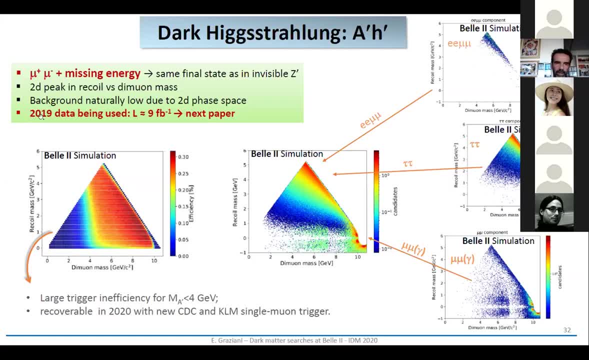 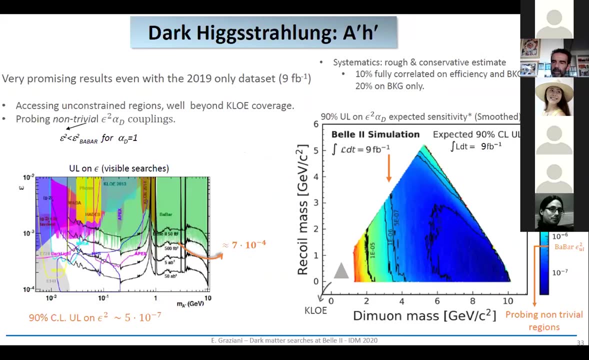 Nevertheless, we decided to use here the single-nual trigger, the 2019 data. so without this trigger, because we already get a very interesting sensitivity just with this small sample and you see here. so these are sensitivity, we get limits, remind you, are in terms of action: square times, alpha. 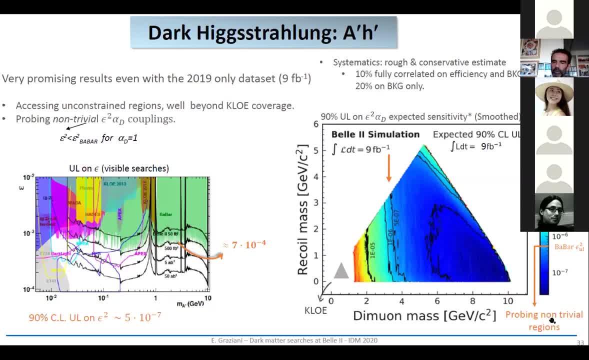 dark. what I mean is a non-trivial coupling, means that if we set, arbitrarily of course, the coupling constant, the dark coupling constant, to one, we get limit in terms of epsilon square, which are better than the best available in this region, which are those set by Baba. but even setting alpha for 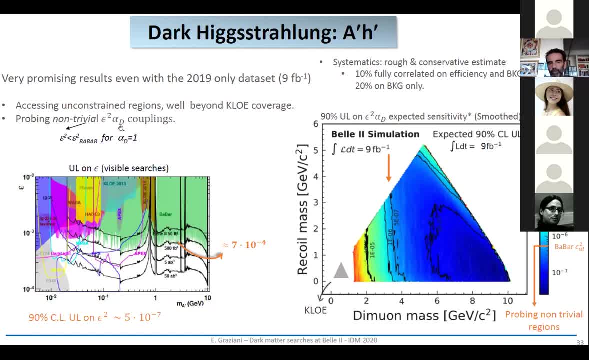 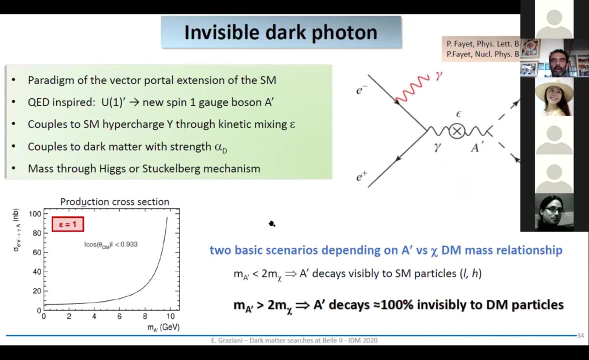 example, to 0.1, 10 to the minus 1, so in the QCD range, so to say. then still, we have a region more or less here where limits in terms of epsilon square are better than okay. so we, I'm going to the invisible. 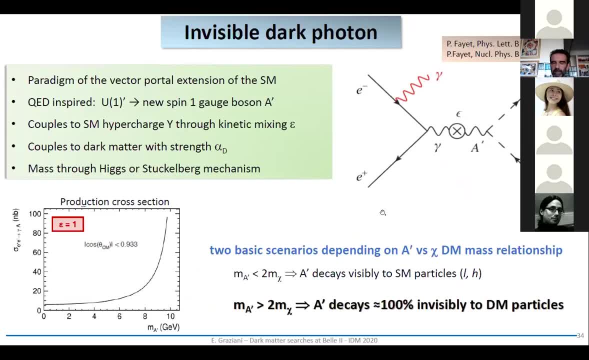 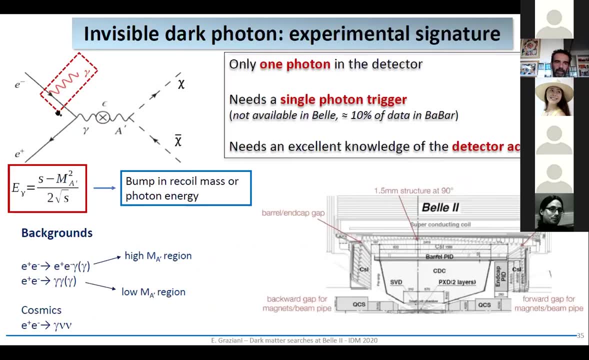 dark photon. so same thing, but this time is invisible, so the only thing that we are left with is photon. we saw examples similarly in LHC, where this can be also object of different nature. of course, this means that a single photon trigger is needed, which was not available in Bell and only partly available in Baba. 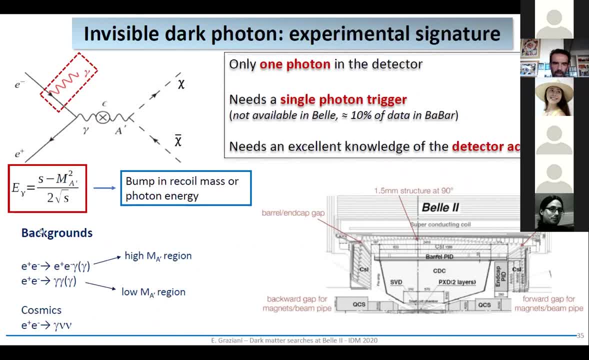 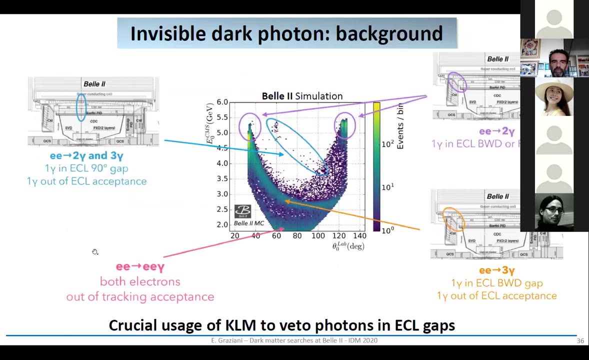 also you need an excellent knowledge of the acceptance, because a QED process can produce photon triggers which, once lost in the gaps, can mimic. the signal signature is a peak in the energy of photon or kinematically equivalent way in the in the recoil system against the against. you see display here how gap we contribute. 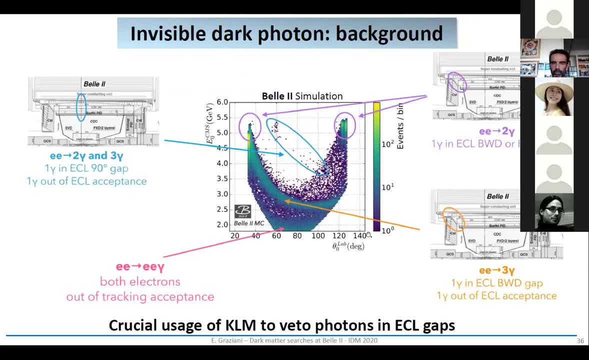 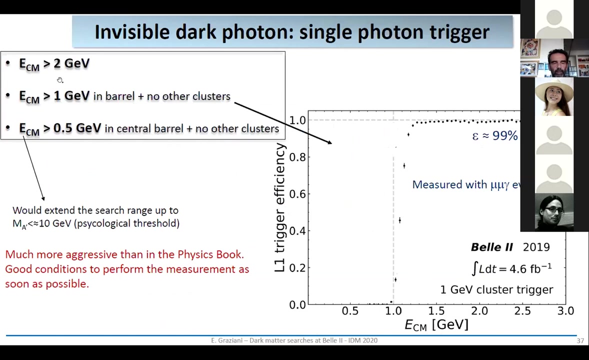 and they produce this funny bans in the two main analysis period which at the energy of the photon in the angle division. so it's crucial to the usage of the muon system to seal the apparatus and to cover the gap, which fortunately do not coincide, which are left in in the character. the main ingredient of this analysis is the single photon. 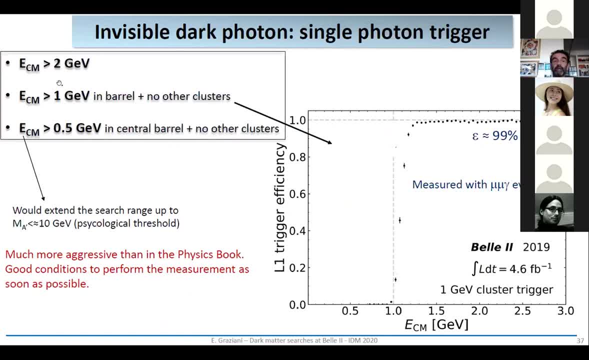 trigger. we have it in three different flavors at the decreasing threshold to one and 0.5. of course, there are other things which are not the same beside the threshold, otherwise we would always use the lowest one. here is an example how the one jet threshold works perfectly in data. this was 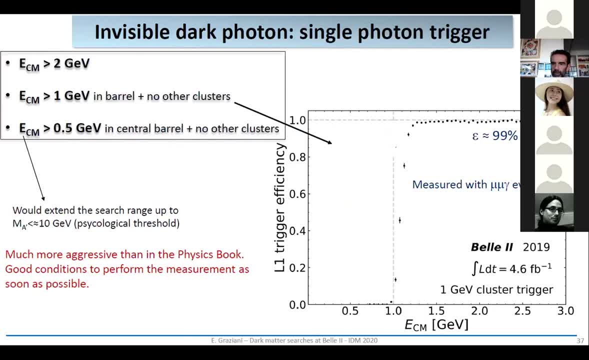 measured with the new program events, wonderful plateau, very close to 100 percent. this is a threshold- the lowest one, 0.5- much more aggressive than what was considered in the physics book. this is an excellent reason to make this measurement as soon as possible using this data, because this: 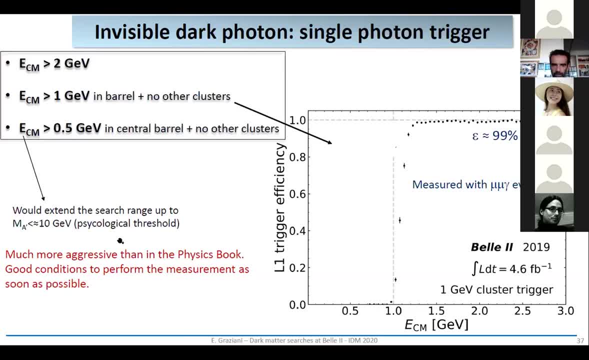 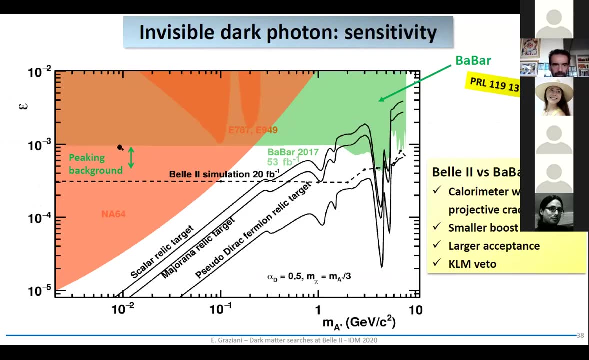 is not guaranteed to survive with increase of luminosity or the country is guaranteed not survive, probably in two years from now. so the word situation now is leaded by by is led by babar, which is a measurement here, and we claim that with the sample, with luminosity more than a factor two less than baba, 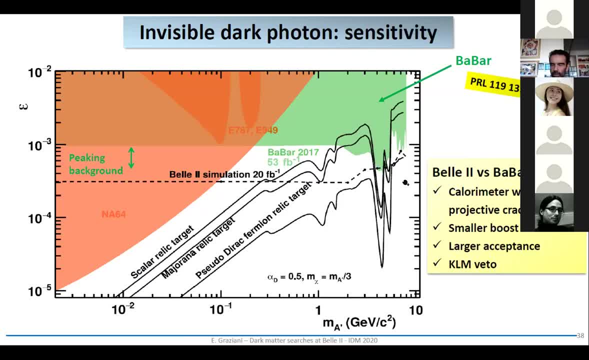 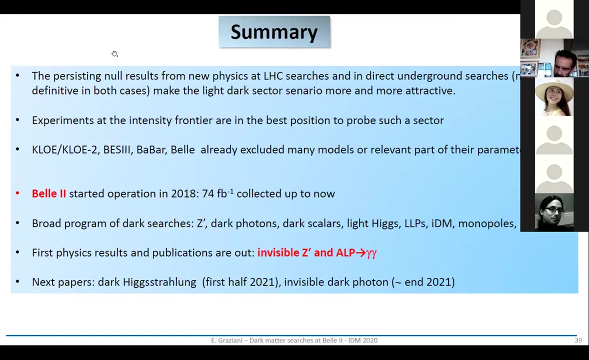 we. we make much, much better and this is due to the calorimeter structure which is not projecting cracks in phi, which means better hermeticity, and also two factors combined, the smaller boost of the machine and the larger kilometer sides, together make a larger acceptance and also the usage of kale. so we will see. i quickly go to summary and persisting new results. 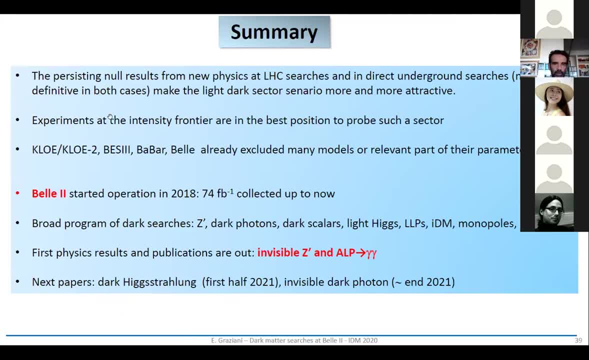 from lgc and the research make more and more attractive the possibility of a light- dark sector scenario. the experiments at intensity frontier are in the best position. there was a great job by chloe 2, base 3, babar and bell, which excluded the full models or relevant. 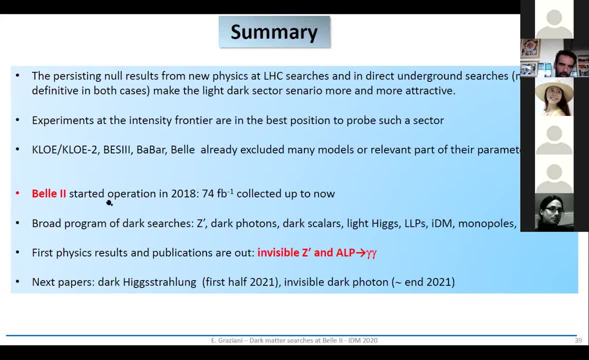 part parameter space of these models and then, jumping to bell 2, started operation two years ago and collected 75 investment of one up to now with the broad program of dark search, much broader than what i showed you today. for example, i didn't talk to you about that. scholars like x.